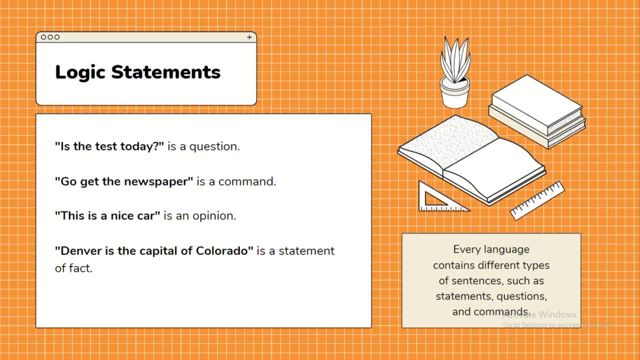 sentence tells something that is true or real. So these four are all types of sentences, sentences, but only the last sentence is an example of a statement. so paano ba natin malalaman? if a sentence is a statement, a statement is a declarative sentence that is either true. 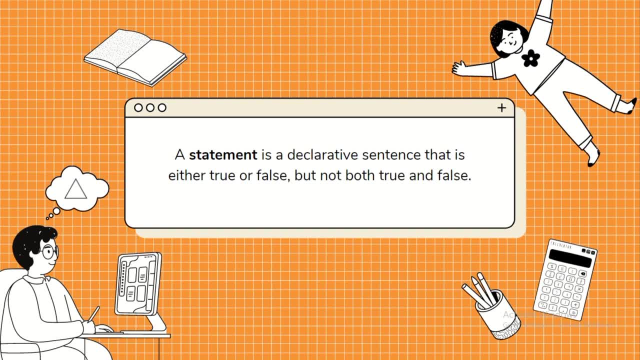 or false, but not both true and false. so ang pinaka indicator to know if a sentence is a statement is kung declarative sentence ba sya o hindi. it doesn't always matter kung true or false sya, as long as it is declarative. pero there are some instances when a declarative 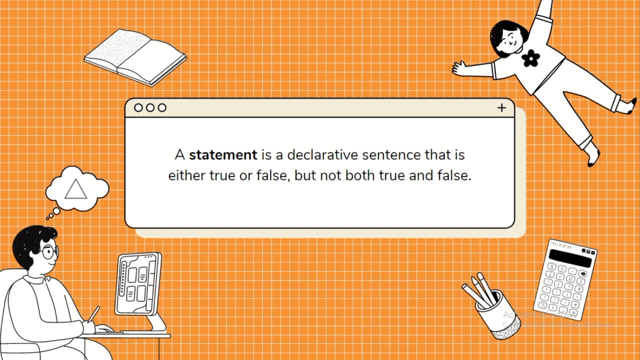 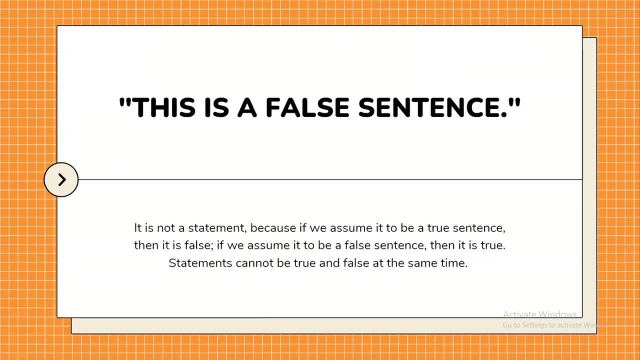 sentence cannot be considered a statement, and that is when the sentence is both true and false at the same time. an example of that is this sentence: this is a false sentence. it is not considered a statement. kasi, if you assume it to be a true sentence, then it will. 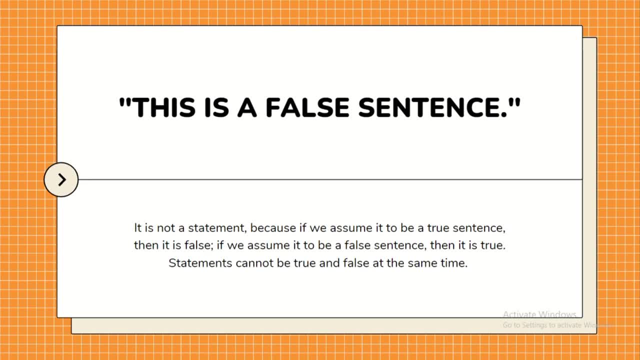 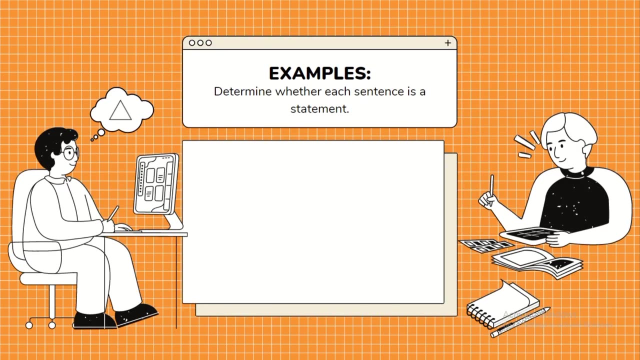 become a statement, false statement but. but if we assume it to be a false sentence, that it is a true statement. remember, statements cannot be true and false at the same time. so for more examples, determine whether each sentence is a statement. number one: florida is a state in the united states. this sentence is a declarative sentence and florida is really. 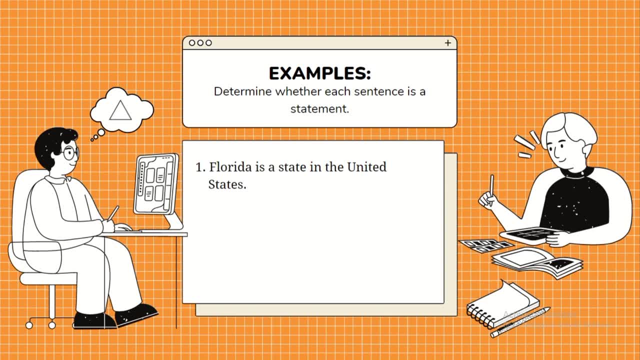 one of the 50 states in the united states making the sentence true. therefore, this sentence is a statement. number two: how are you? this sentence is not a statement because it is a question, therefore not making it a declarative sentence. number three: nine raised to nine plus two is a. 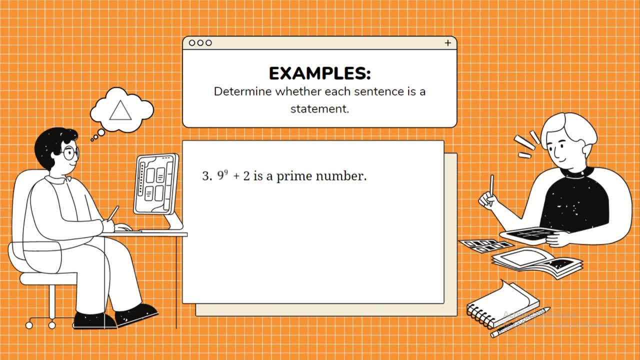 prime number. so this sentence is a declarative sentence and even if we don't solve it, we do know that the answer can either be a prime number or not. a prime number meaning the sentence can either be true or false, and not both true and false. so therefore this sentence is a statement.